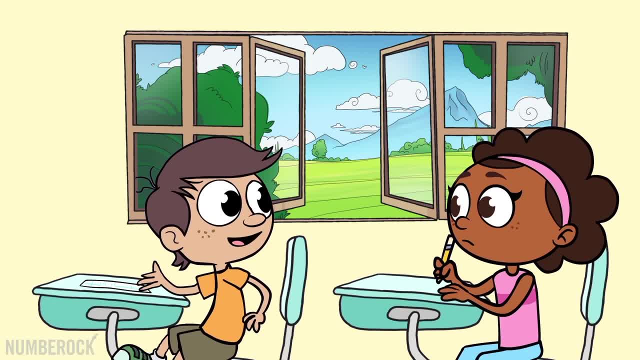 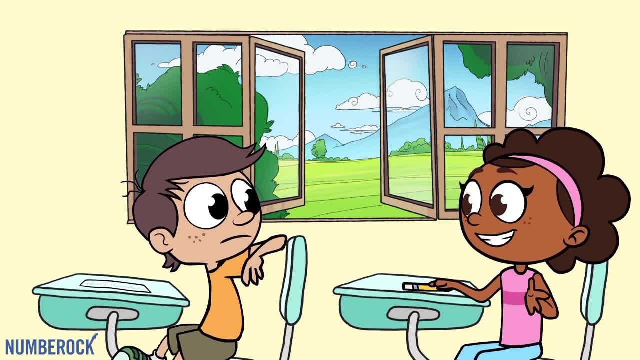 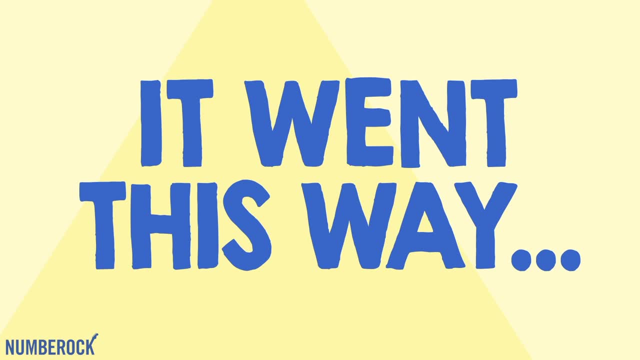 I asked my friend: do you ever wonder how to convert an improper fraction to a mixed number? She said: actually, my brother showed me how to do that yesterday. Then she sang a song. it went this way, It went this way, it went this way. 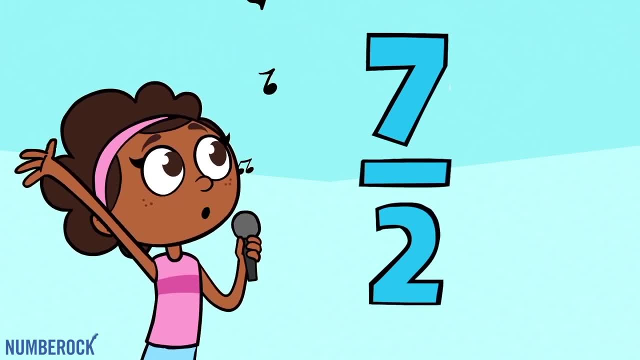 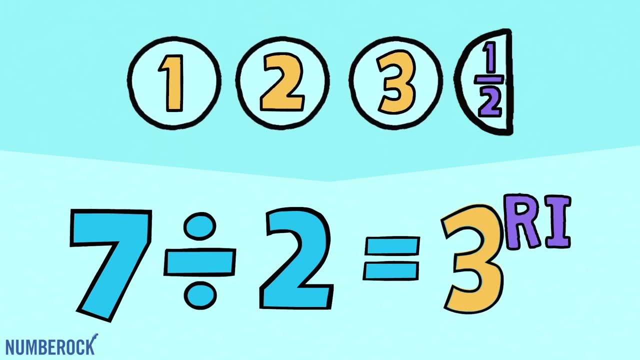 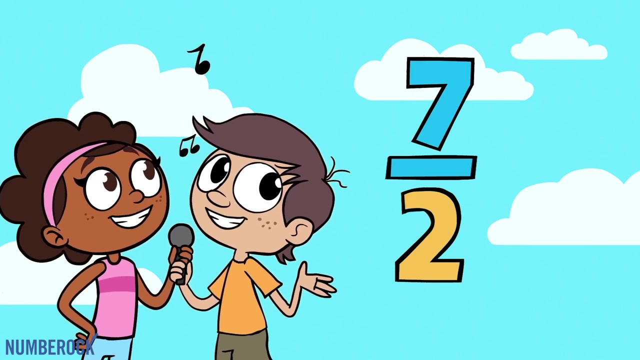 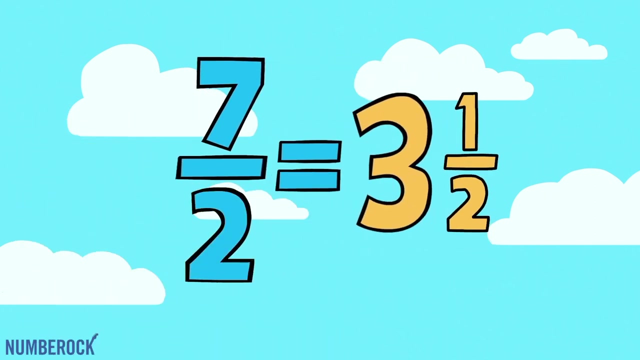 When there's an improper fraction to convert, divide the top by the bottom and then insert The remainder as the numerator, the divisor as the denominator. An improper fraction has a numerator that's greater than or equal to the denominator. A mixed number has a value that is greater than one. 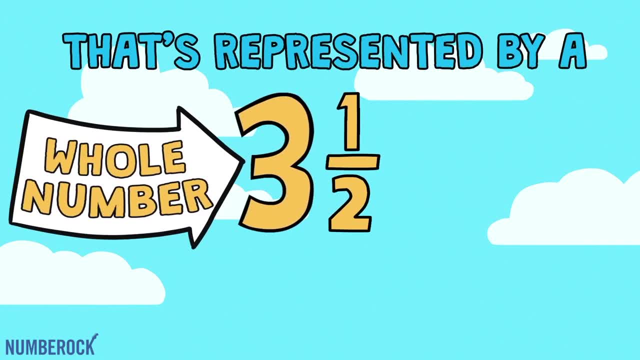 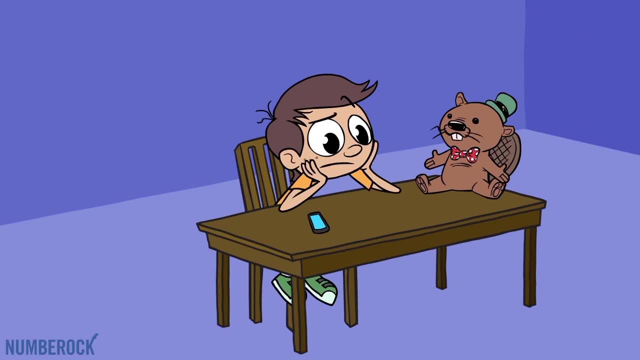 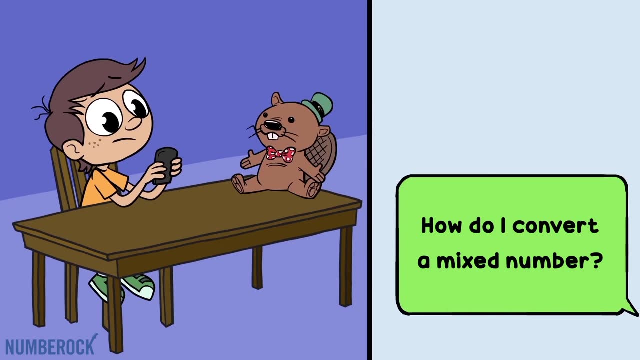 That's represented by a whole number and a fraction. There was a mixed number that I had to convert. I thought so hard my brain started to hurt. I texted my friend for some more advice. She sent me this song. it was clear and concise. 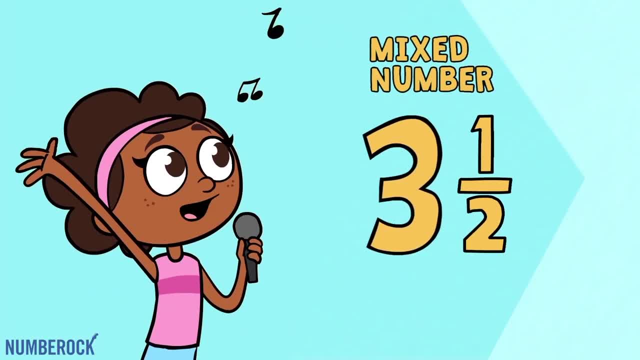 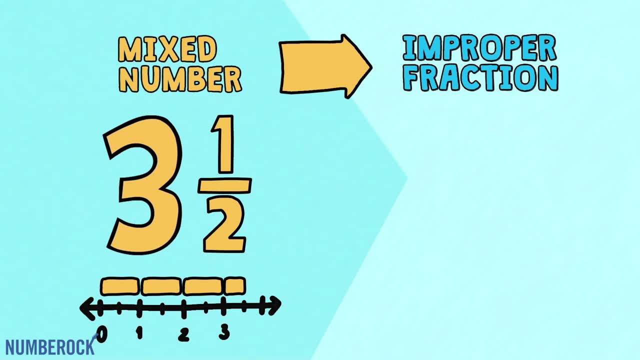 So clear and so concise. To convert a mixed number to an improper fraction, three simple steps will give you that satisfaction. Multiplied. Multiplied the whole number by the bottom, then add to the top, keep the denominator the same and then let the beat drop. 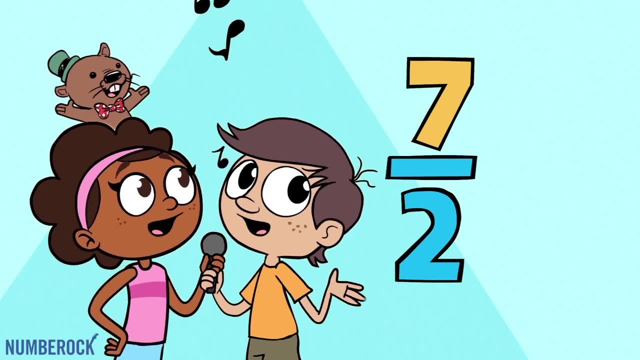 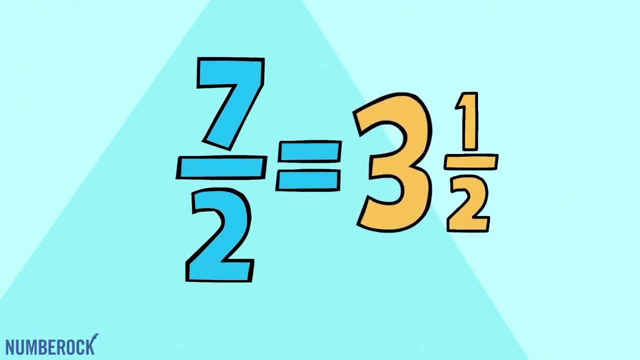 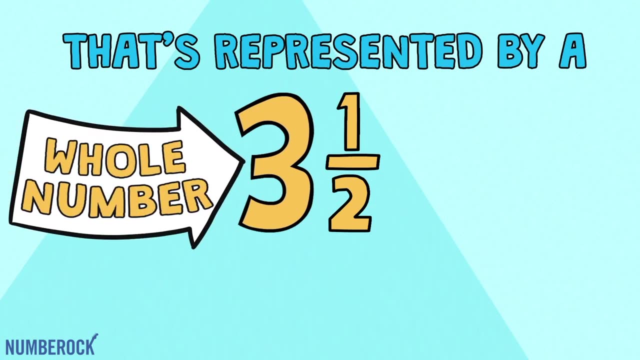 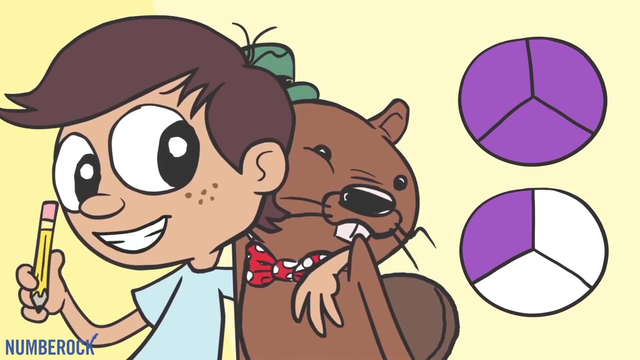 An improper fraction has a numerator that's greater than or equal to the denominator. A mixed number has a value that is greater than one That's represented by a whole number and a fraction. Oh yeah, Let's take a look at these circles and describe the amount that's purple. 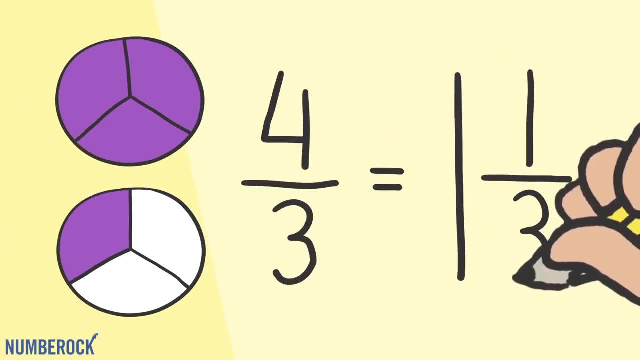 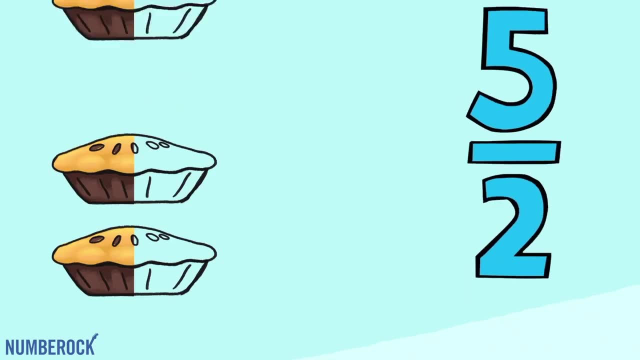 It's four thirds, so we could write four over three, but one and one third seems a little clearer to me. Converting to a mixed number makes sense when describing the amount a value represents. For instance, consider five halves of apple pie. Two and a half seems easier to visualize.